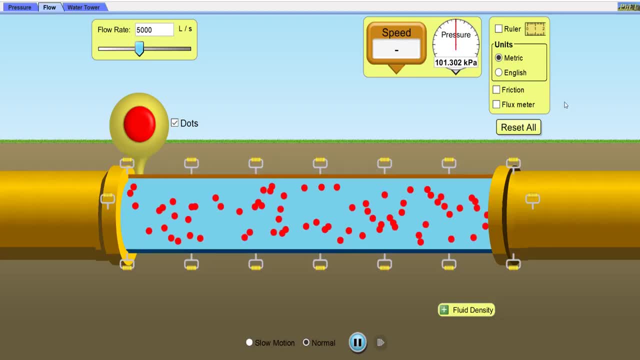 Hi, I'm Lalit Vasist and you are watching Engineering Made Easy. In this beautiful simulation of fluid dynamics, we will learn various concepts like what is equation of continuity? We will measure the speed and pressure of this fluid at various points. We will also vary the flow rate of this fluid and we will add friction to it. We will see it without friction and we will add friction to it. 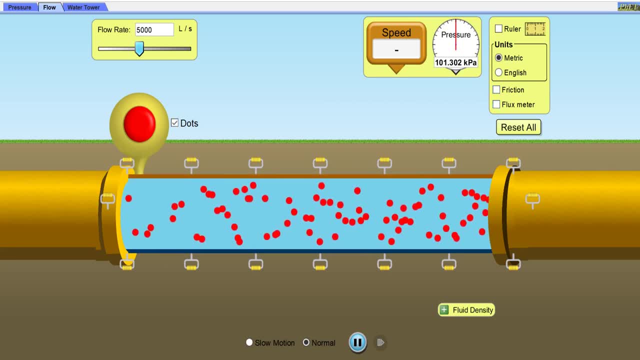 By adding friction to this fluid. Okay, we will also vary the fluid density and we'll see how it affects various parameters. We will also learn here how the velocity of the fluid is affected when we change the cross sectional area of this pipe. So let's see all these concepts by this demonstration. So we will start with the equation of continuity in fluid dynamics. 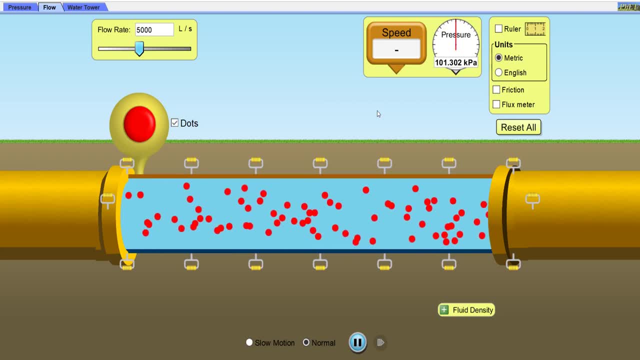 So what we mean by the equation of continuity? It tells us that the product of area of cross section and the velocity is constant for a fluid to flow. It means if we decrease the area, then the velocity will be increased, And if we increase the area, then the velocity will be decreased. You can understand it with the help of a simple, practical example. 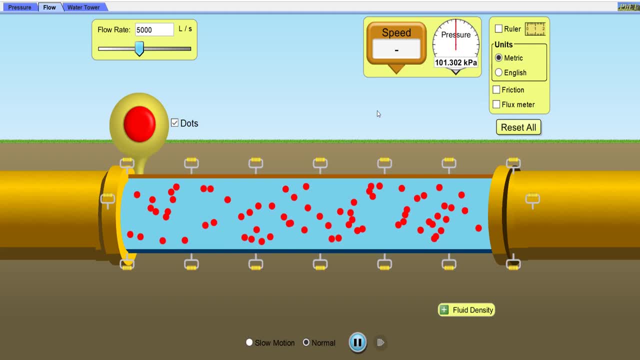 So we have a pipe that has water flowing out of it And if we press the pipe then the water will come out from the pipe at higher speed. So we have reduced the area of cross section of the pipe, then its velocity increased. This is nothing but the equation of continuity. It means area into velocity is constant. It is nothing but simply the law of conservation of mass. 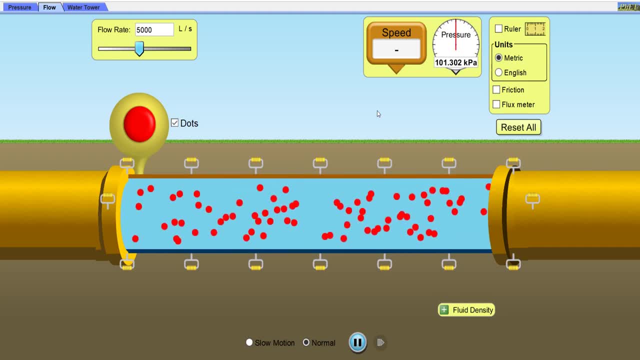 For a fluid to flow, it must conserve its mass. So let me show you how it happens. Look at this. Here I have a pipe and fluid is flowing through it. So let's understand it. by changing the shape of this pipe, I will reduce the area at some places, while at other places I will increase its area. You observe the velocity, how it affects. 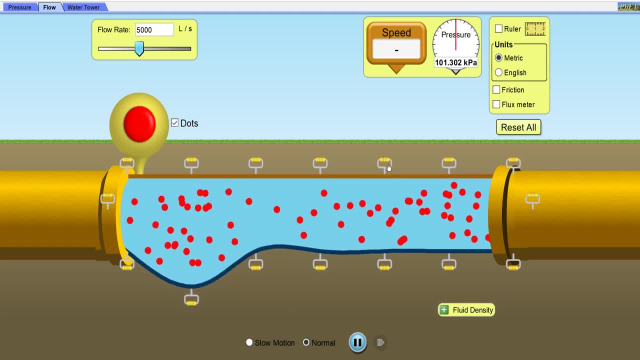 Increase this area and at this place I am reducing the area. I have reduced the area at this place. Now you can easily observe that at the place where the area is large, the velocity is small, Velocity is less, And at this place, where the area of cross section is less, the velocity is high. 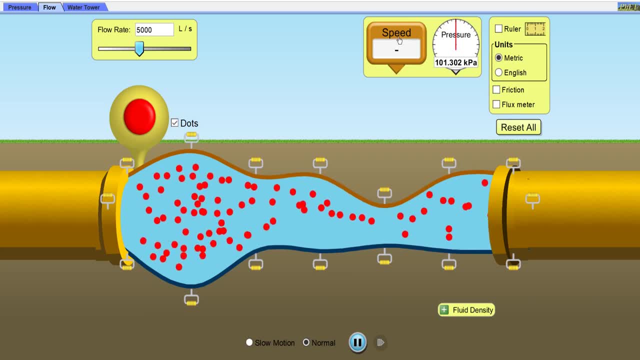 We can also observe it. with the help of this speedometer. You can measure the speed and the direction You see here. here it is showing. this arrow is showing the. what is this? This is a vector. It is showing the direction. Its direction of arrow is showing the direction of the fluid and fluid particles, And the magnitude is shown by its length. So it's 0.5 meter per second at the place where the area is. 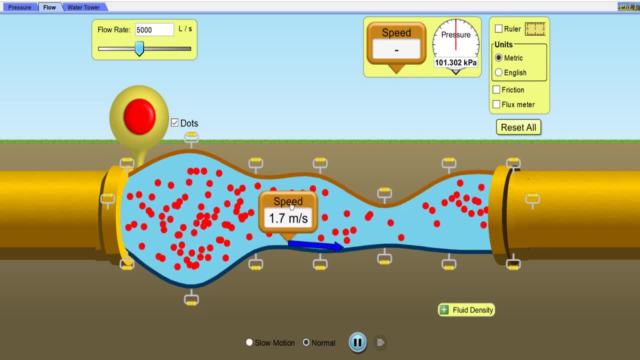 Large, Let's move it towards smaller area. You can observe it by its magnitude, that its value is 5 meter per second, and the length of this vector, blue vector, showing its magnitude, that it is much higher in comparison to at this place, where it is 0.5 meter per second, And here it is 6 meter per second, 6.1 meters per second. So this is the law of. 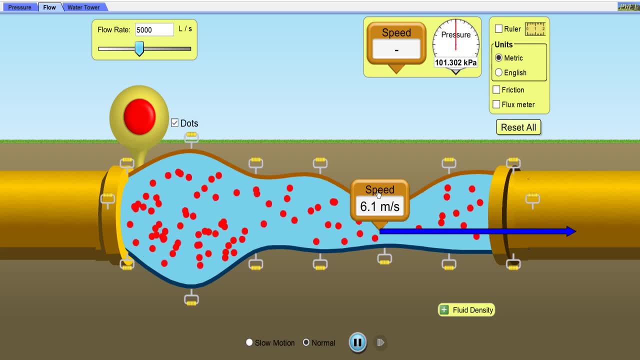 continuity, the equation of continuity in fluid dynamics, which says that if I increase the area, like this, then its velocity will be reduced, And if I reduce the area then its velocity will be increased. So the product of area and velocity is always constant in this flow of fluid. This is the law of mass conservation, because the amount of mass that is 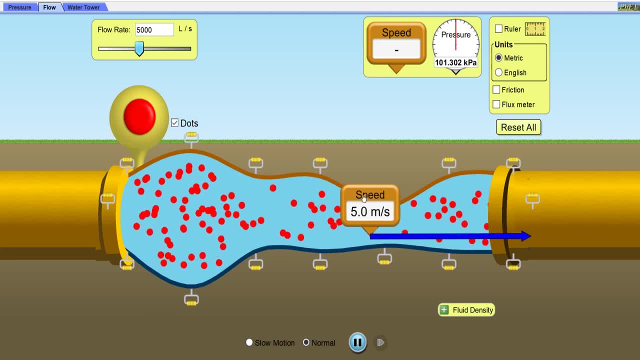 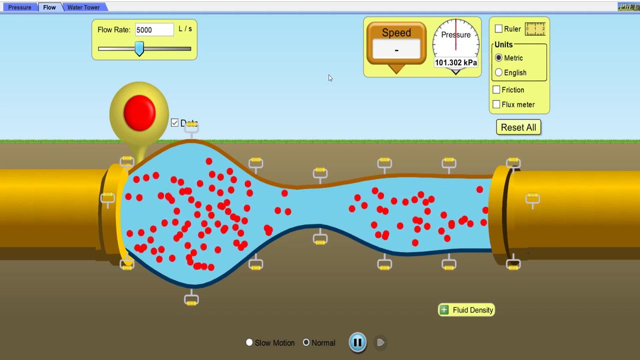 entering from this end must come out at the other end. Okay, So the mass is conserved. If I have larger area for the fluid to flow, then it must flow at lower speed so that the law of conservation of mass is followed. Okay, You can more clearly visualize this equation of continuity by this thing that I'm going to show you Here. I'm pressing this button. 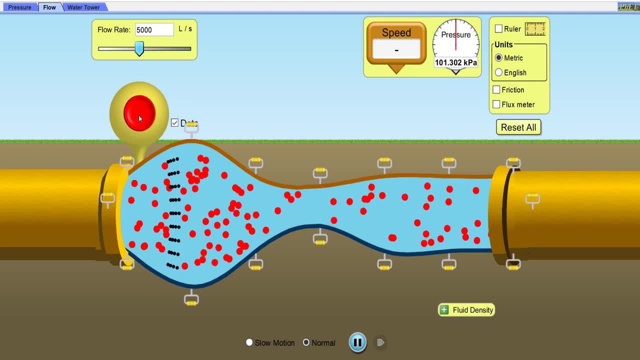 And you see few dots. You observe its motion, that they are moving at very small speed at this place And as it passes through this constricted area that is a small, smaller area, its motion is, its velocity is increased. You observe here it is moving at low velocity, very low velocity, And as soon as it passes through it it moves at fast rate. Okay, So this is nothing but the. 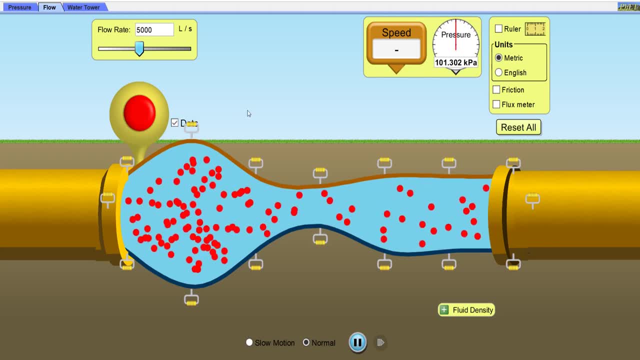 equation of continuity, that is, area into velocity, is always constant. Okay, Now I will show you one more concept related to the pressure of the fluid. According to Bernoulli's theorem, if there is a horizontal flow of fluid through a pipe having varying cross sectional area, then, according to this, the pressure is reduced at the places where the speed or the velocity 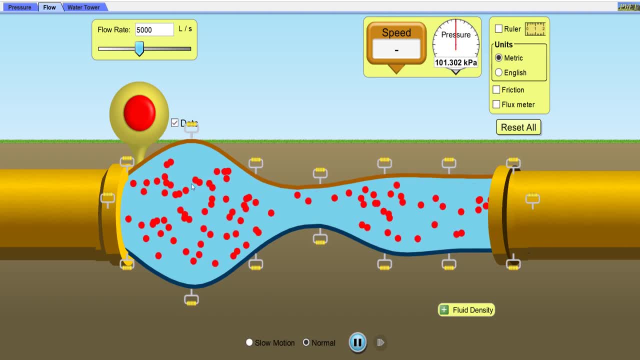 of the fluid is high. So at the place where I have larger area, that is, the velocity is low, its pressure should be high, And at the places where the velocity is high, the pressure should be low. So let's measure it. You see that at this place we have a smaller velocity. So the area, so the pressure, is 122.579 kilopascal. Okay, 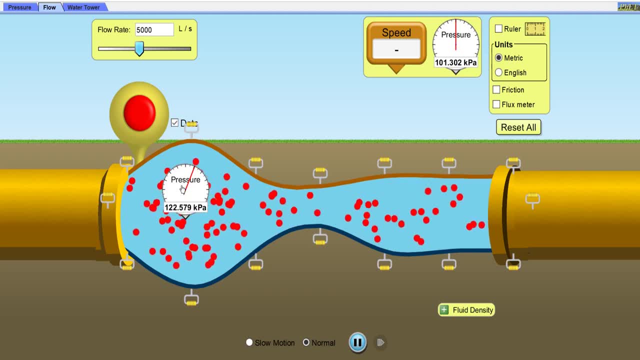 Pascal is a unit of pressure, So you remember 122.5.. Okay, And at this place, as I move at this place, it becomes 101.. Okay, it has reduced because the velocity of the fluid is high at this place. So as I'm moving towards the particles having lower velocity, the pressure is increasing: 110113.. You see 117113.. 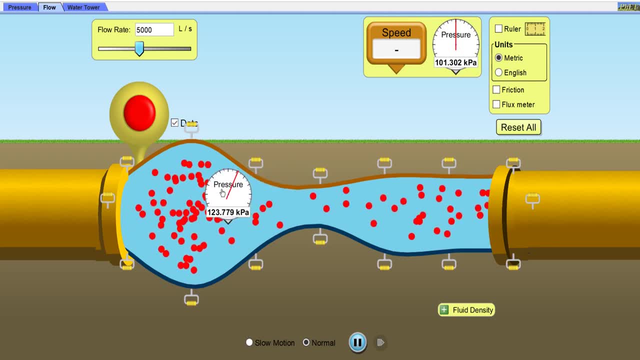 118,, 120,, 121,, 22.. And in this way, 124.. Okay, And as I move at this place, the pressure reduces. it proves Bernoulli's theorem, according to which, actually, Bernoulli's theorem will be discussed in another lecture, where I will dedicate the whole lecture for the Bernoulli's equation- we will learn how it affects the velocity pressure. it is actually the law of conservation of energy, while the 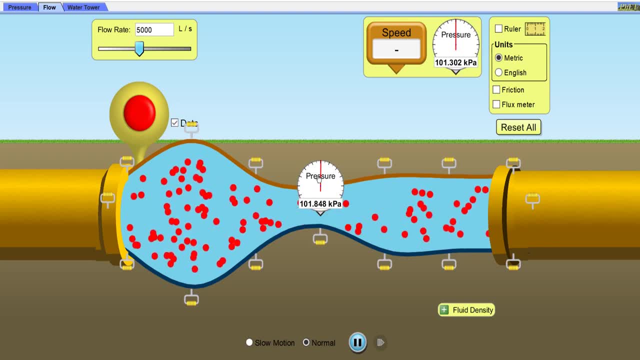 equation of continuity that we have just seen is the law of conservation of mass. So this was mainly dedicated to the law of conservation of mass. that is the. that is the continuity equation. In next video lecture I will show you what is the Bernoulli's equation. Okay, we will see it. So I hope you liked the video. And we can also vary various parameters. Let me change various parameters And we will measure its. 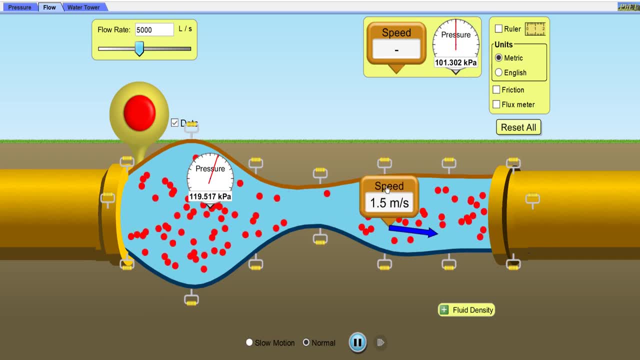 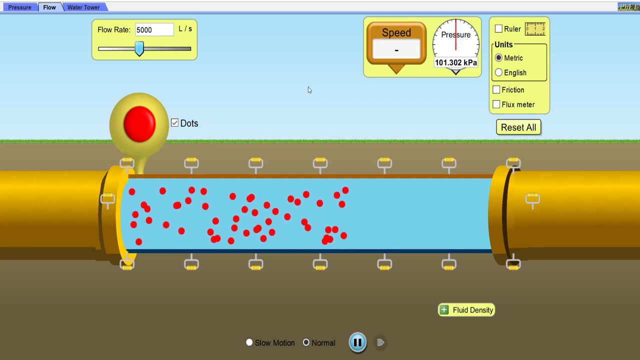 speed and pressure at various points by varying the area of the pipe. Let's change the friction. Okay, I will show you the friction, how it affects the motion of the particles of fluid when I add the friction. Okay, let me first reset it. Okay, to the normal shape. Now I will add few dots. you see the velocity of these dots, Okay, 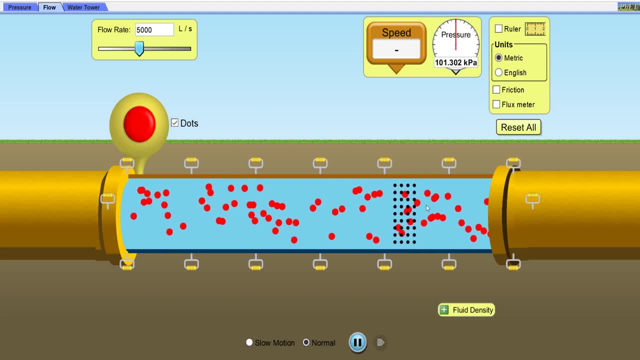 are moving very smoothly. okay, you see here, now i will add a friction, some friction to this. now see, friction has been added. this is the shape of these dots. you see, it is resisting the motion of the free flow of these particles of fluid without friction. its motion was like this: 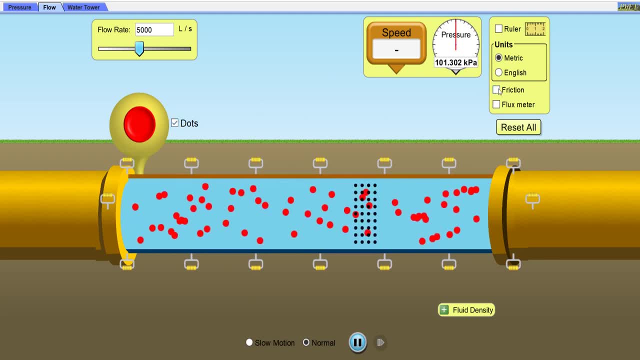 okay, but when i add friction from this into this, then its shape will be something like this: observe the motion of these particles, dots. okay, and we can also change the flow rate from this. okay, we can increase the flow rate. okay, its velocity will be increased, we can. 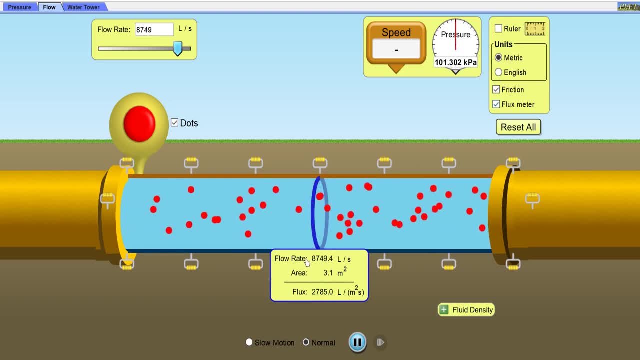 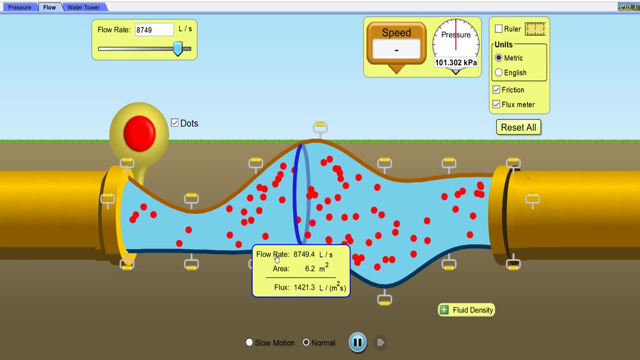 add the flux meter to it. flux meter is what it change. it shows the flow rate in liters per second. okay, it would be better to change the shape so that you can get better idea of it. okay, you see, if i observe it, then you can say: you can see here that the area here is 0.8 meter. 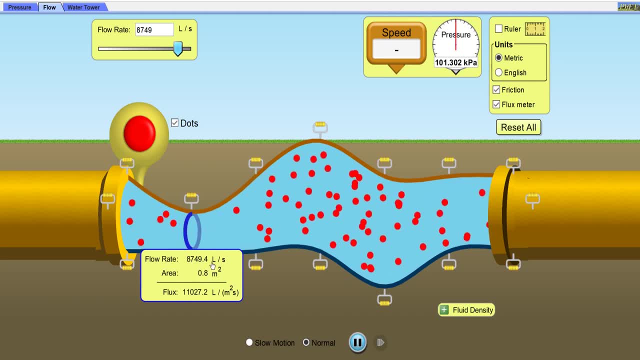 meter square and the flow rate is 87 4749 liters per second. flux is what flux is Denoted as the flow rate divided by area. you see liter per second divided by meter square. So how much fluid is flowing through this cross-sectional area per second?